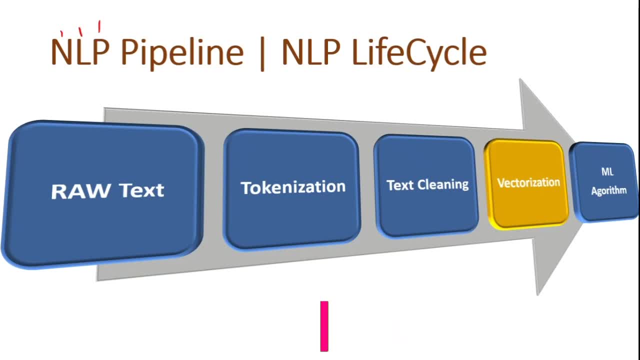 intelligence. It comes under artificial intelligence And this field uses language, computer science, information engineering and artificial intelligence. Natural language is a language in which human interacts with each other. Natural language processing: it's a related with the interaction between the computer and the human languages. In NLP we will train computers or 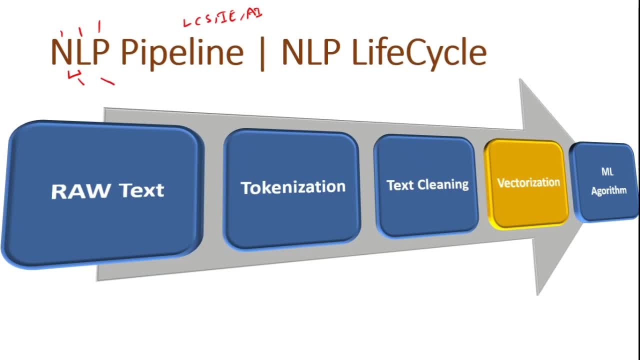 machines to process and analyze large amount of natural language data sets, So that data could be in form of text and speech, audio, anything It would be natural language As considering NLP. it's a process. This process has several steps And I have listed down the 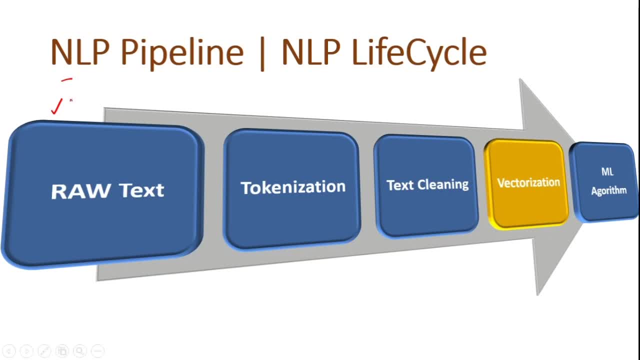 information in the description box. So let's start. So NLP is a natural language processing important step. So first is raw text. So raw text is generally that we will get as a data set. So it's a first step. It would be raw data. We have to extract information from the raw data. So in 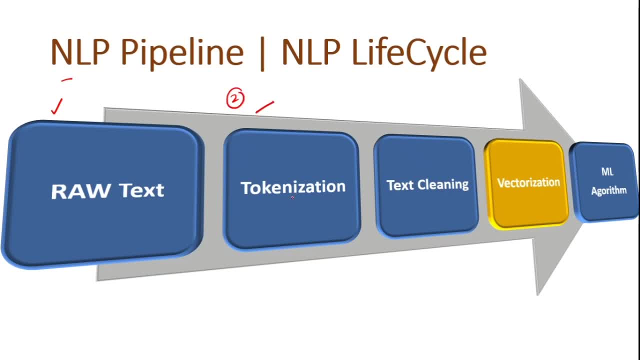 second step, we will perform tokenization. So tokenization is a process in which we will create a tokens from the raw text. So in this first we will convert the paragraph into sentences, And once sentences are formed then we will create a tokens, or we can say it as words. So first, 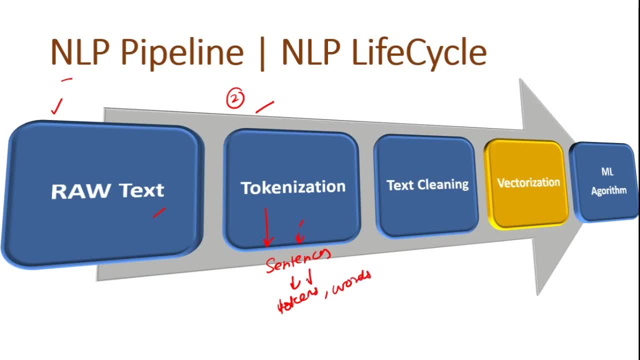 we will convert from paragraph to sentence, then sentence to words, Then after we will perform text cleaning, And in text cleaning there are several process. We will perform stemming, We will. we can perform lemmatization. These are the same thing. If we will perform stemming, then we will. 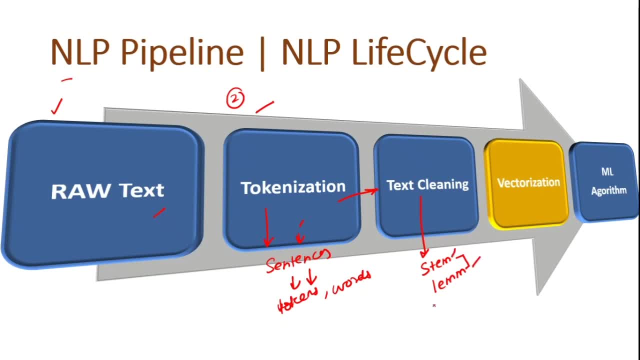 performing lemmatization. So these are the same thing And we will remove stop words. So basically, stop words are like a and the, I, we. So these are the stop words. We will remove these stop words. We will remove punctuation. 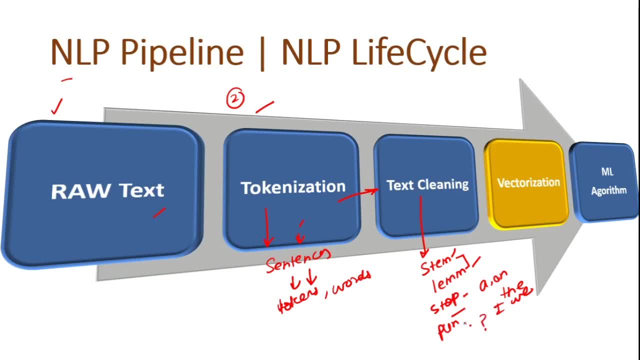 Basically comma full stop question mark. So we will remove punctuation, We will convert uppercases into lowercase character, We will remove the URLs, We will remove apostrophe s and we will split attached words which are attached together and we will standardize words. Suppose someone has. 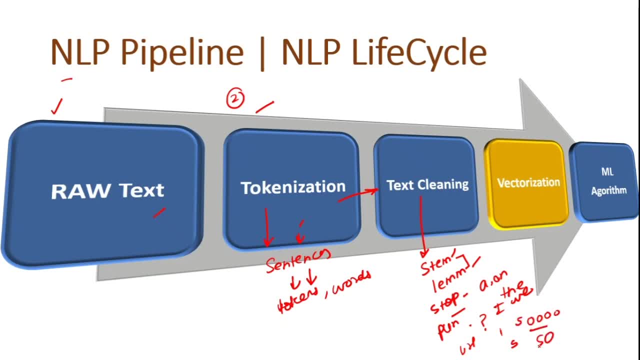 written a so like this. So we will remove extra out and we will convert to into so and we will decode the data into standard format. Once we have cleaned the text, then we will perform vector vectorization And basically we will talk about vectorization in this video. So vectorization is 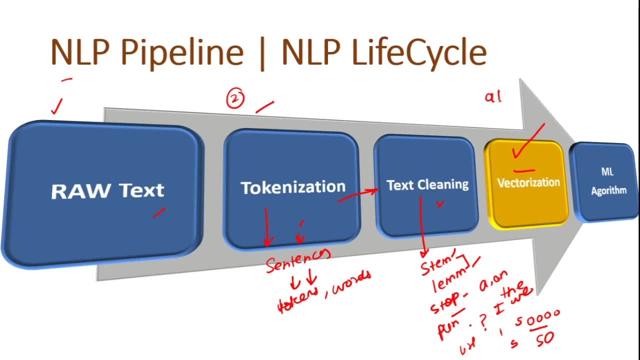 just a converting alphabets into integers, So I will show you in further slides. So as of now you can take it as we will convert characters into numericals And once we have the numbers then we will apply ML algorithm. And this ML algorithm it could be for any applications like we can perform. 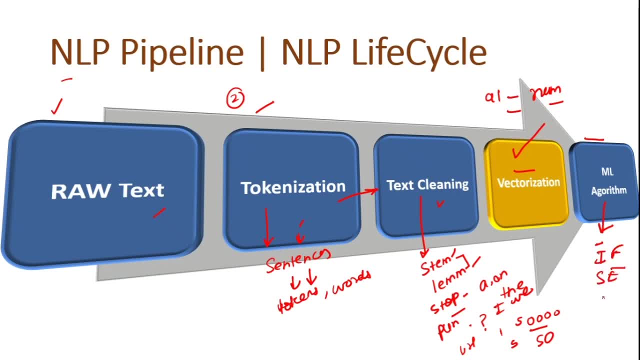 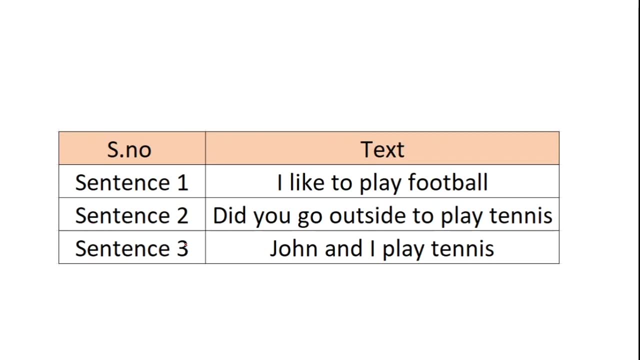 information extraction, we can perform sentiment analysis, we can perform spamming, we can perform spam detection or we can perform language translation. So here I'm taking a very simple example to just get a better clarity of this step. So suppose we have a three sentence. This is our. 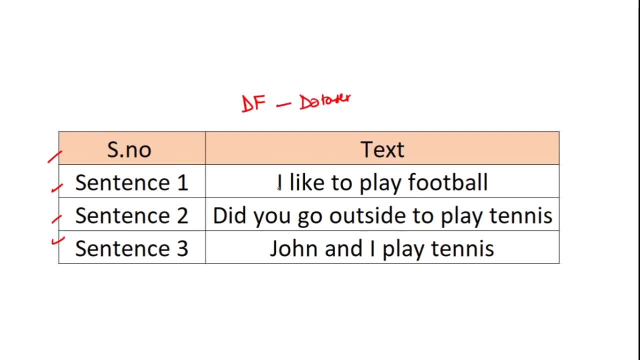 data set. This is our data set, or we can say data frame. in this we have three sentence: I like to play football. Did you go outside to play tennis, John, and I play tennis. This is our raw data. This is raw text. So, first step, we will perform tokenization. So tokenization I have already. 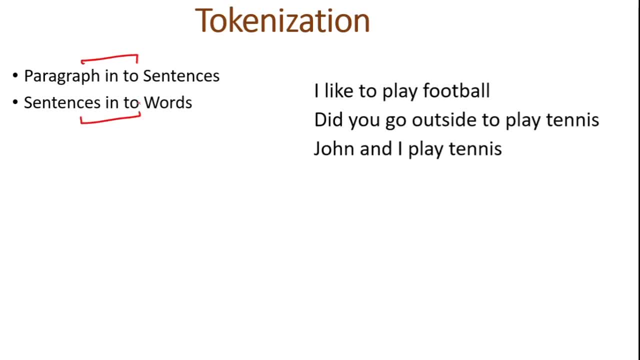 explained. We will convert paragraph into sentence and sentence into: So this is our data. I like to play football. Did you go outside to play tennis, John, and I play tennis. These are my sentence. Sentence one, sentence two, sentence three. So I have converted. 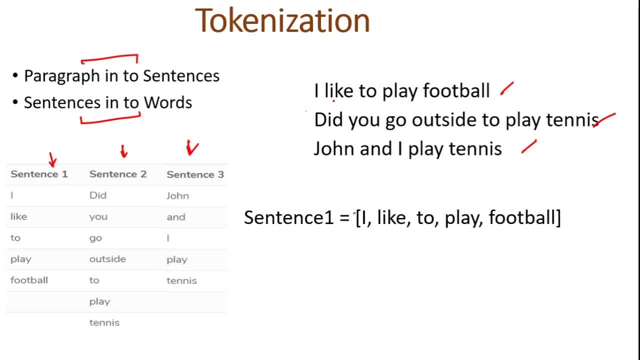 paragraph into sentences And now I will convert into tokens. So sentence one has converted into tokens one, two, three, four, five. So this is a list. This is a list of strings in Python. So this is sentence one And by this it will be sentence two and sentence three. So my tokenization is: 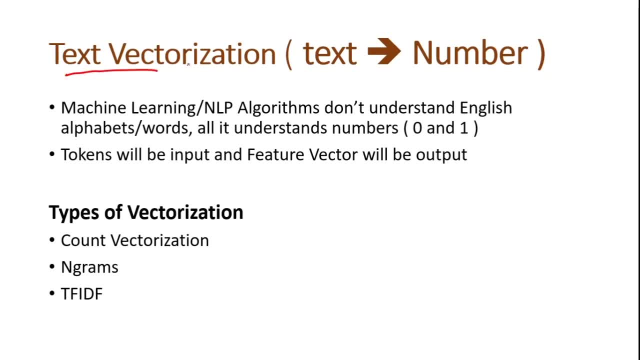 completed, So now I will perform text vectorization. So, first of all, why do we need text vectorization? As we all know that we have to convert categorical values into numerical values in machine learning algorithms, Because machine learning algorithms don't understand English alphabet or categories. Machine learning algorithms understand numbers. 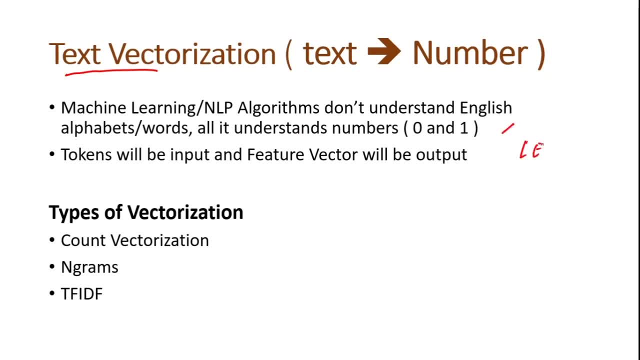 which is zero and one. So what we do in machine learning, we use label encoding, We use one hot encoding or we use get dummy, So that all processes converts categoricals into numbers. So, but in NLP it could be one lakh text, But in machine learning we generally have two, three or four or ten. 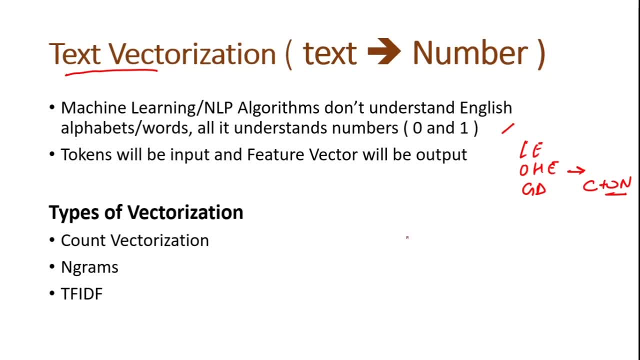 categories at most. But in NLP there are many categories And all these categories are just words, English words. So we won't be able to perform these things. So in NLP we will perform text vectorization. So text vectorization, it would be algorithm. So this would be an algorithm. 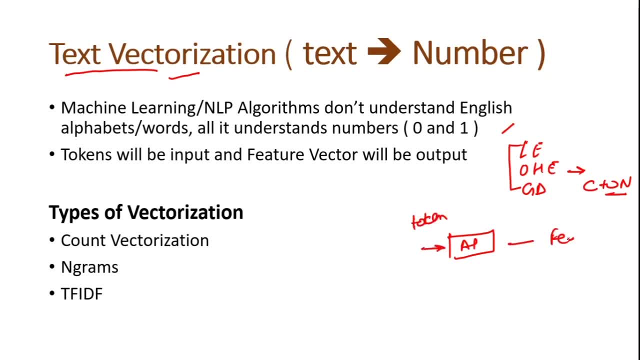 in which input will be tokens and output would be feature vector. So output would be feature vector. So in NLP it would be numbers numerical form, Here it would be alphabet form, word form And here would be number form. And we have many types of vectorization techniques. So in this video 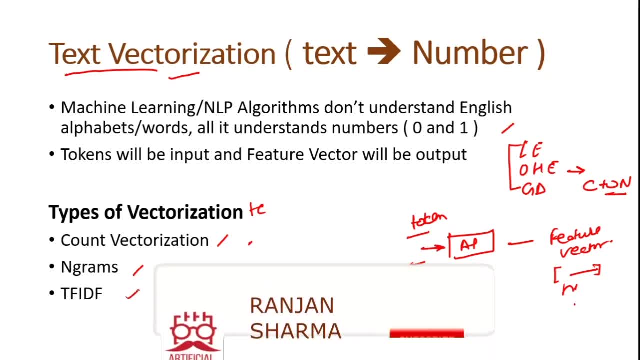 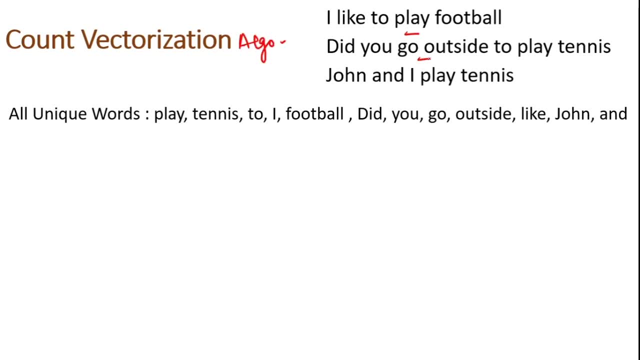 we will talk about count vectorization And we have ngrams, tf, idf, say term frequency, inverse document frequency. In this video I am talking about count vectorization algorithm. So this is our data set. We have three sentences and we have already created tokens And from: 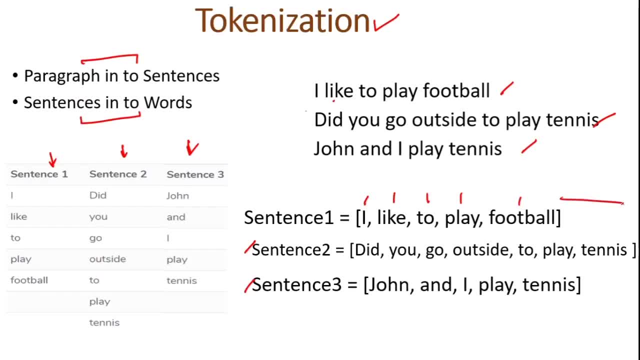 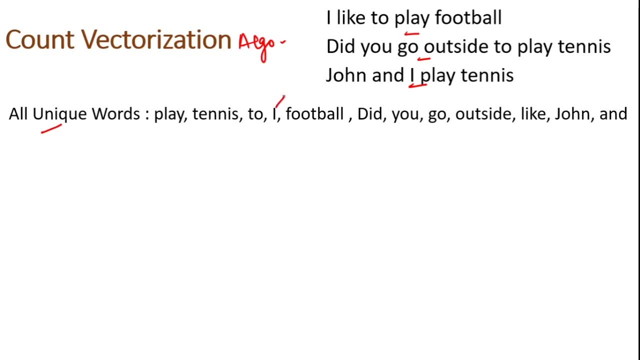 the tokens, I will select unique words. So from all these words I will select unique words Here. you will see I has come twice, but I will write I only once. So I have written I only once. So these all are my unique words. Now what I will do: I will create a new data frame. 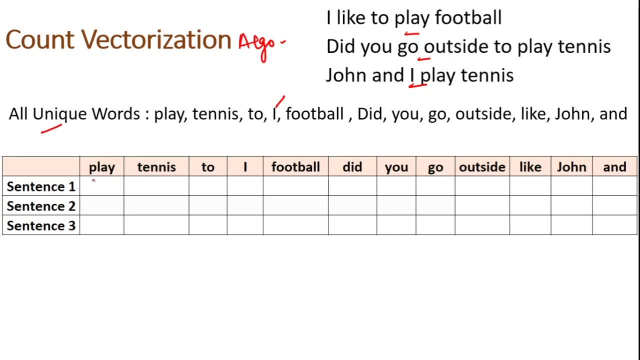 because I have to write numbers only in that data frame. So I will write like this: So these are all my unique words. So I have written like this and these are my sentence one and sentence three. So what I will do I will just see. like in sentence one play word comes how many times, So play word. 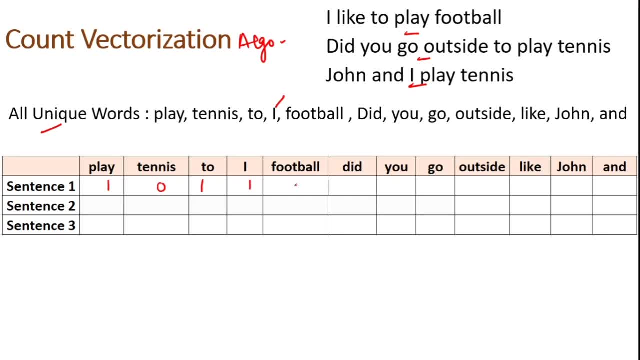 one and tennis, zero to one, I one. and football, one did zero, you zero, go has not outside, no, outside, yes, low, like zeros on and zero. and so same is with this play, yes, tennis, yes two, yes, I zero. football zero did zero, zero did is one and you is one, go is one, outside is one like zero, Sean is zero and 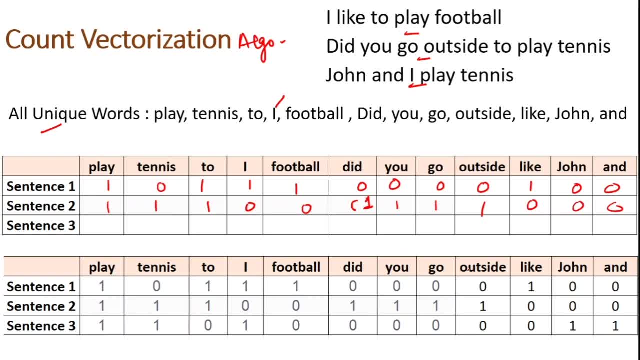 is zero, So it will be like this. So now we have created a data frame which we have only one and zero. It could be any number, Suppose in sentence when football is coming twice, So we will write two here. So now. now our previous data frame was looking like this: 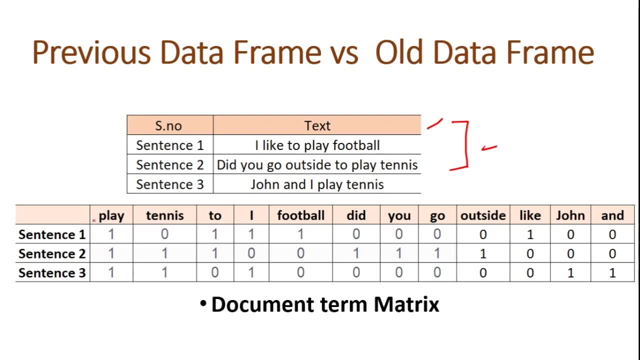 has alphabets, It has words, And now we have converted into this data frame, It would be new, previous data frame and new data frame. This was my previous data frame And now my new data frame is looking like this And we generally call this as document term matrix. So this is count. 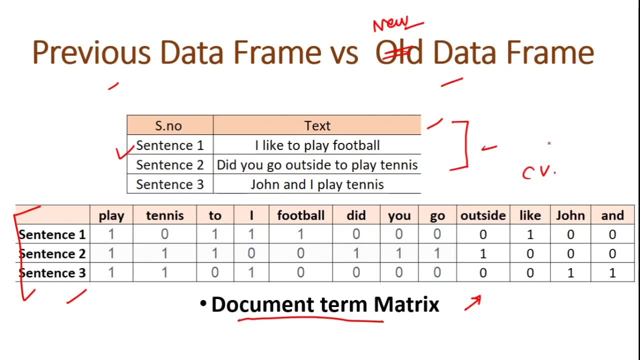 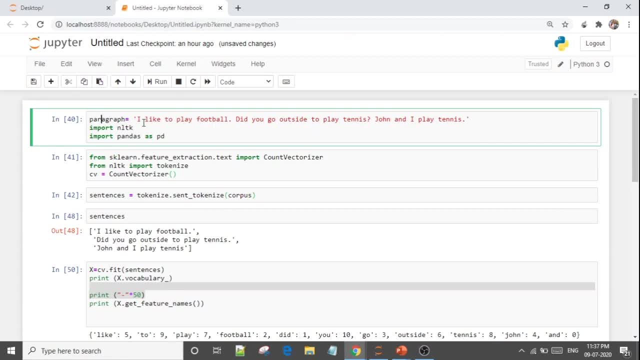 vectorization. So now, this was a theory. Now I will perform the implementation in Python. So this is the same example that I have explained. I am taking that example. This is my paragraph, and in this paragraph I am taking example same: I like to play football. Did you go outside to play tennis? and, John, I play. 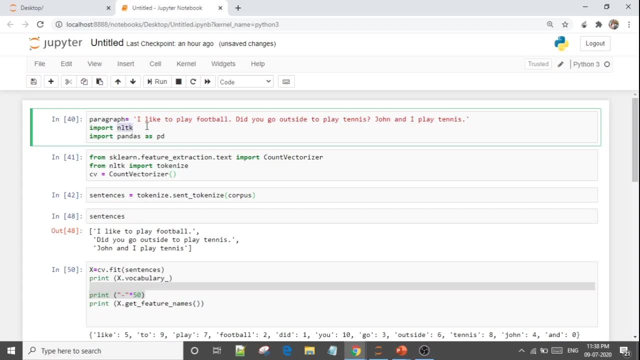 tennis. So this is my library, which is NLTK. If you are using this first time, you have to install by pip. install NLTK: This is natural language toolkit and this is pandas, which we were using in machine learning as well, And this is count vectorization, which we have just seen. 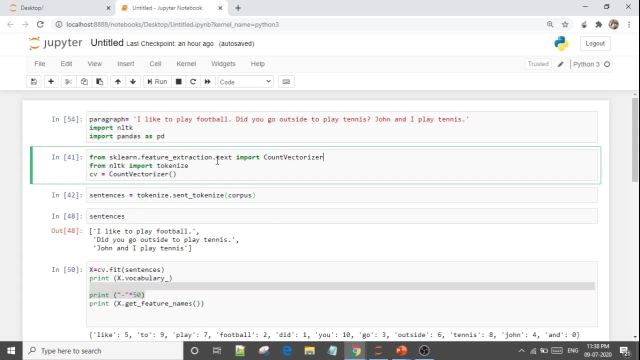 And this algorithm is comes from the sklearn feature extractiontxt and from the NLTK. I am importing tokenize. here I am creating a shortcut for count vectorization as CV. Now I will convert paragraph into sentence. So here you will see. these are my sentence And now what I will do. 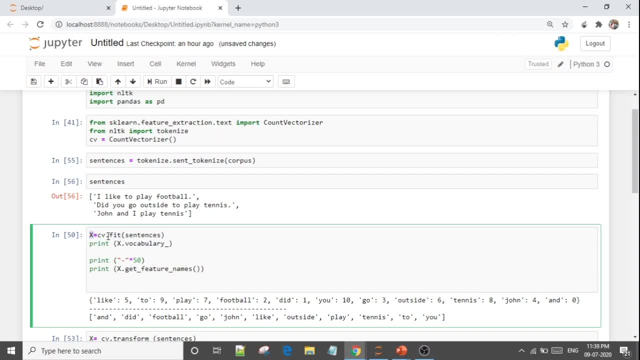 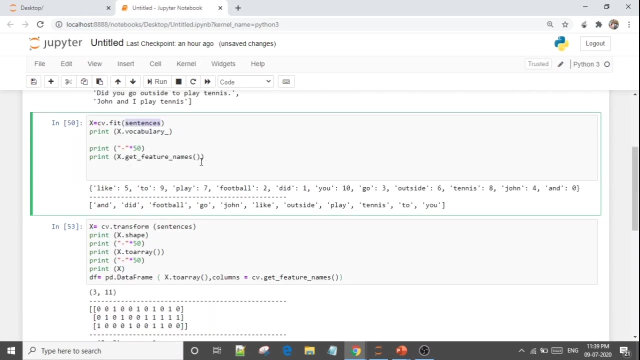 here I'm creating a X variable and I'm using CV, which is my count vectorization, and I'm using fit and inserting sentence in this. If you will see, I am typing X dot vocabulary underscore And you will see like it is creating like this. So it has written all the unique variables, If you. 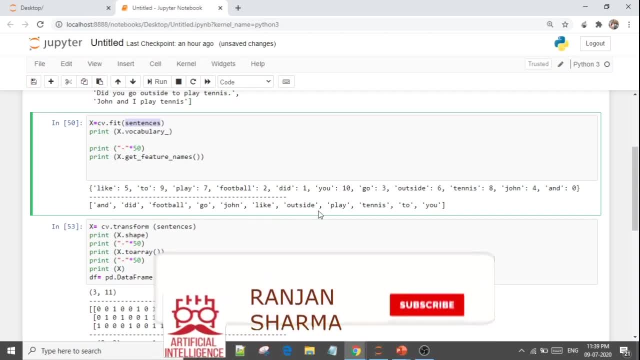 will see that. and did football go, John, like outside play tennis to you? This all are the unique variables that we have listed down in our theory And this, this number is like, it is pointing to the position. If you will see, here is and, and, and comes at zero, and zero, and it is one, So it is one. 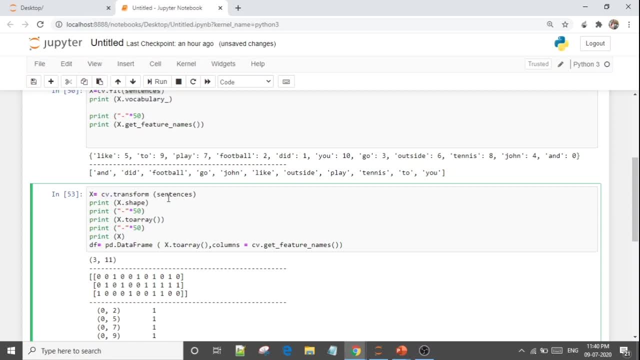 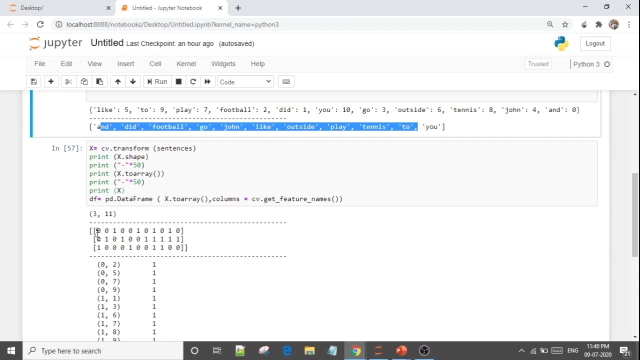 CV is my count, vectorizer and transform. I'm using a non sentence, So my X will be having a shape of three dot eleven, five, three, because I have three sentences: This one, this one and this one and 11. 11 is my unique variables, So it comes like this, And earlier it was not an array, So we have just 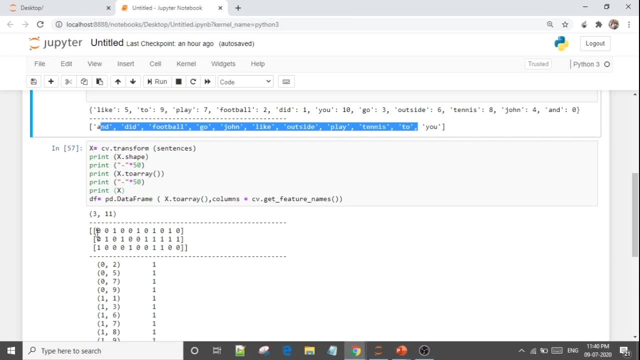 converted into X dot two array. Here it is coming like a array, So it is coming in an array form or a matrix form. This is sparse matrix. We called it as sparse matrix And here I have printed all the things. This will show me only once at which position it is one. So this is. 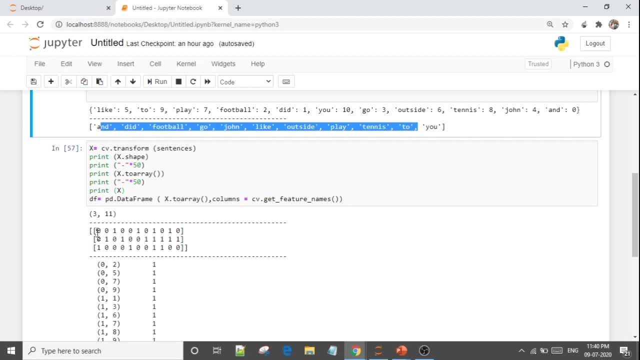 zero row and this is second column, which is one, and you will see zero five, So zero at five finite. to print the data frame for this, I will use period or data frame and I will use X dot two array and columns. I will use features name, which I have written in the above set. So here you will see it.